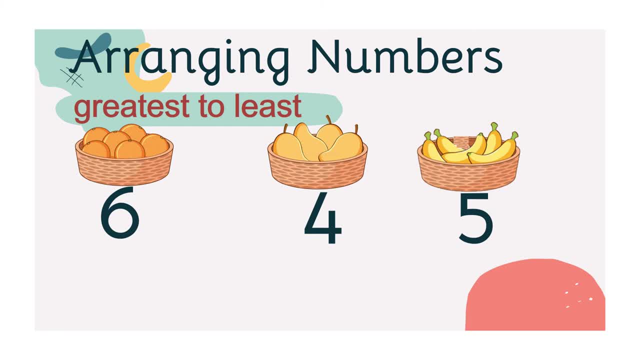 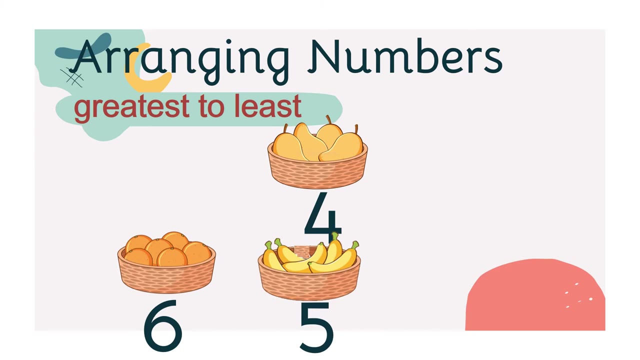 Now let's try to arrange numbers from greatest to least. So the greatest number, or the biggest number, is 6.. Next we have 5. And the least number is 4.. So if we are going to arrange the numbers from greatest to least, 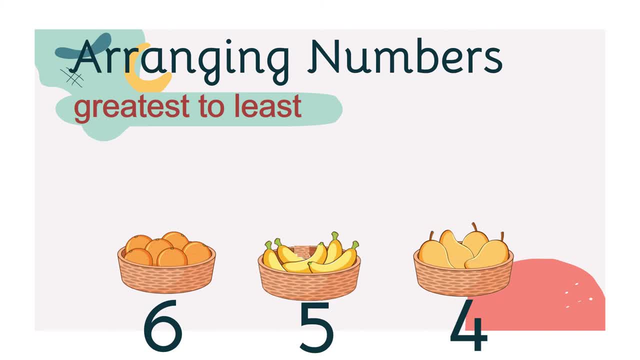 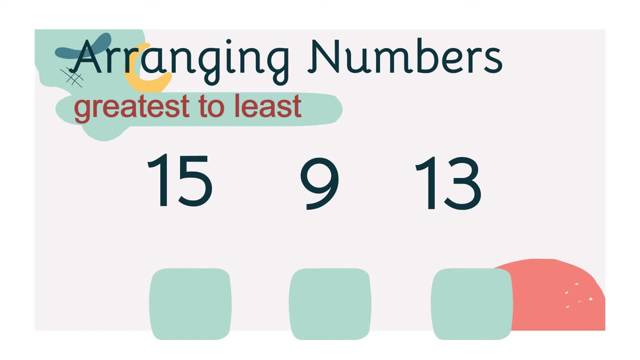 If we are going to arrange the numbers from greatest to least, arrange the numbers from greatest to least, we have six, five and four. how about this? let's try to arrange them from greatest to least. which number is the greatest or the biggest value? will you point on the screen? okay, number 15 is the greatest number. how about the next number? 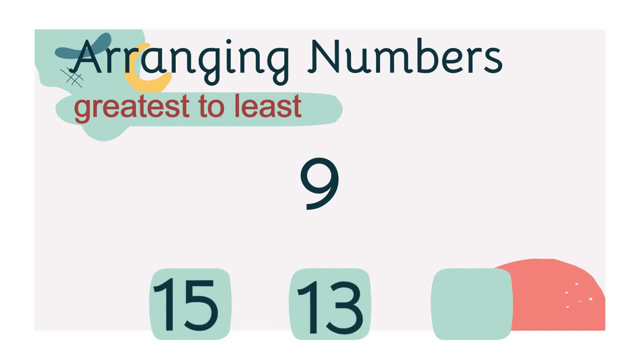 very good number 13. after 13, the list number is number nine. good job. if we're going to arrange them from greatest to least, number 15 comes first, then 913 and then number nine. next. let's have this number: seven, five and nine. which one is the greatest number? good job. number nine is the 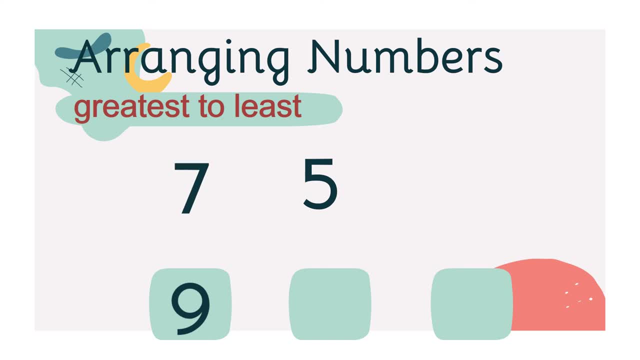 greatest number. how about the next number? very good, number seven. and the list number, great job, number five. so we have nine, seven and five. and last, let's arrange these numbers from greatest to least, which are 14, 20 and 16. which one is the greatest number? 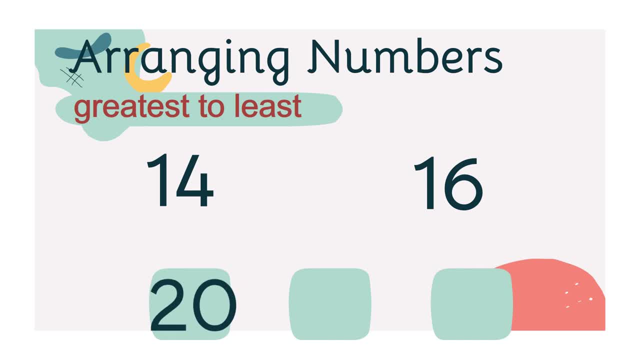 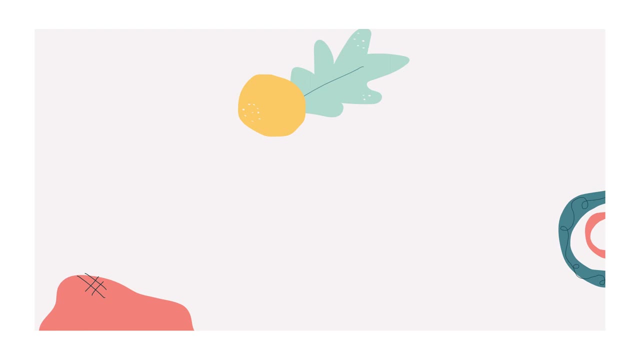 very good, it's number 20. how about the next number? very good, it's number 16, and the list number is number 14. great job, and let's have a review. so what did you learn today? great job, you learned about arranging numbers, and we arrange numbers from. 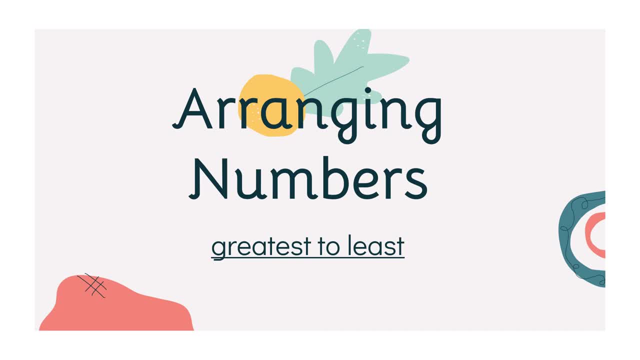 greatest to least. kids always remember that when we arrange numbers from greatest list, the biggest number comes first. okay, the biggest number comes first. okay, it comes first okay. So I hope you learned today. See you on our next lesson.